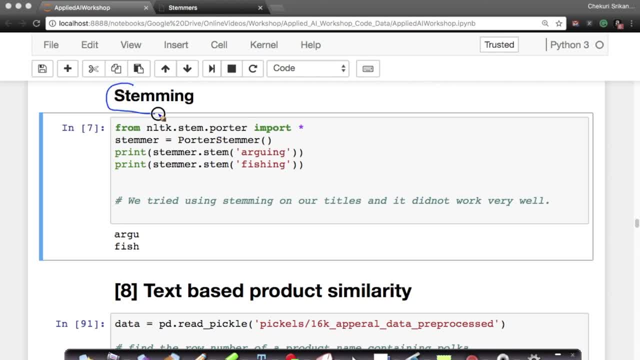 Another very popular text preprocessing system is called stemming. So we saw stop word removal. there is something called stemming. Let me explain you what stemming is. Suppose if I have words like fishing, fisher and fished, All of them are more or less talking about something. 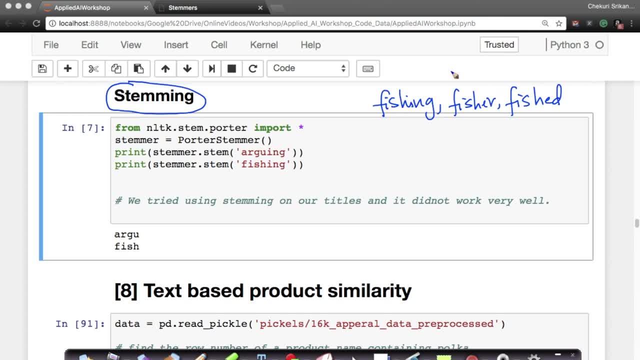 about fish. So all these are related to the word or the root word called fish. So this is called the root word. Similarly, if I have words like arguing or argument, if I have words like this, all of them have a root word which is argue. Again, remember there is no e here. 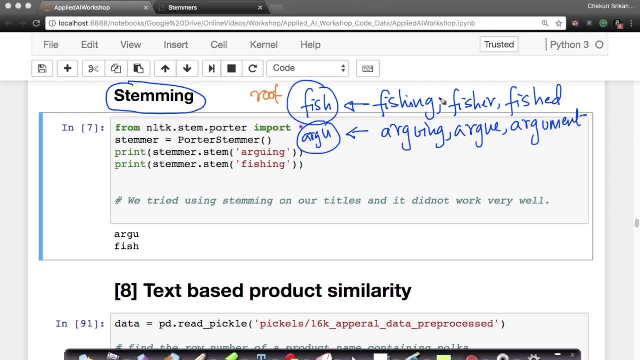 So this is the root form and these are all the various forms of the same word. So when you have words like this for some natural language processing systems, for some types of text processing, it is useful to convert each of your words to their root form. 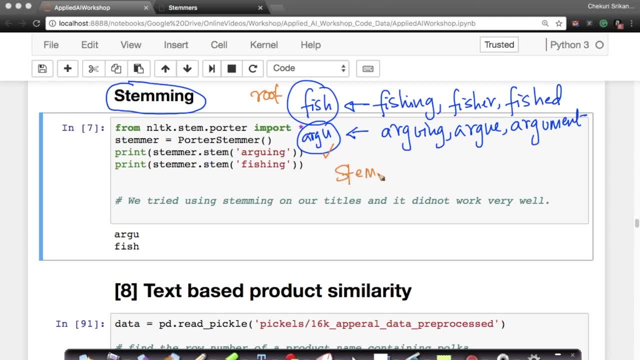 So this is called stemming. Stemming is basically taking a word and converting it into its root form. So whenever you have arguing, you replace arguing with stemming. So whenever you have argument, you also replace with argue, or wherever you have the word fisher. 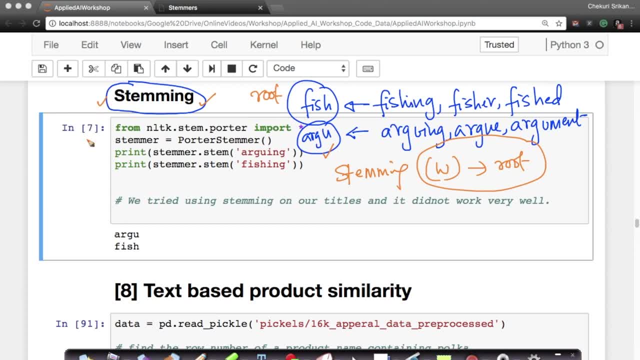 you replace it with fish. So stemming is sometimes useful, and let us see how to do stemming with NLDK. It is very, very straightforward code. So what you do is you basically import something called a potter stemmer, which is a very basic. 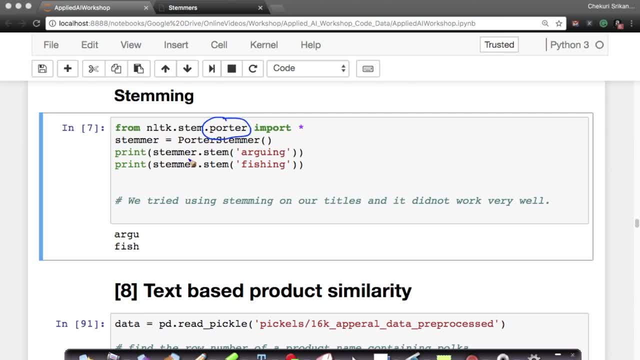 stemmer. There are multiple algorithms to do stemming by the way in literature, in AI research or in natural language processing research. The simplest of them is something called a potter stemmer. So from NLDK I can import it and I declare a variable called stemmer and I declare. 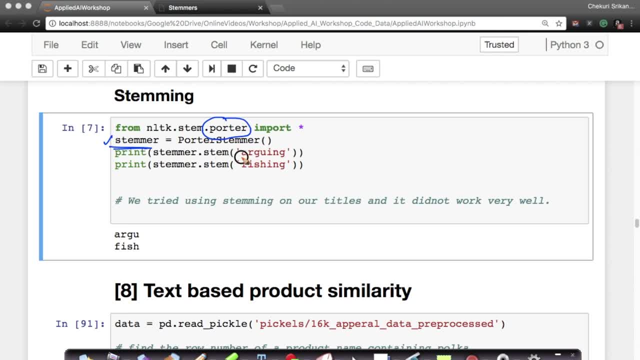 it to be a potter stemmer, and then I just have to say stemmerstem and whatever For this word: arguing. thus, the root word is argue. For this word fishing, the root word is fish. This is how you can do simple stemming. I just wanted to show you some simple code so that, if needed, in other